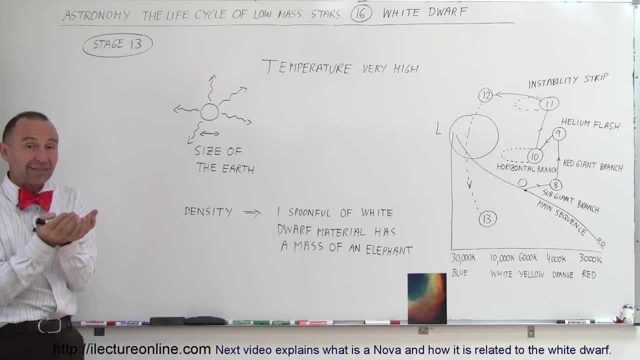 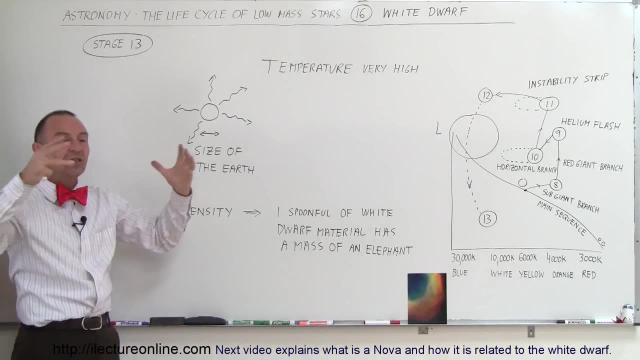 stopped any further collapse. So now we have a white dwarf star, which is basically a ball of carbon, very, very hot carbon, at very high temperatures. Remember, when the star finally reaches its end stage and the outer layers blow away, at that point the core temperature. 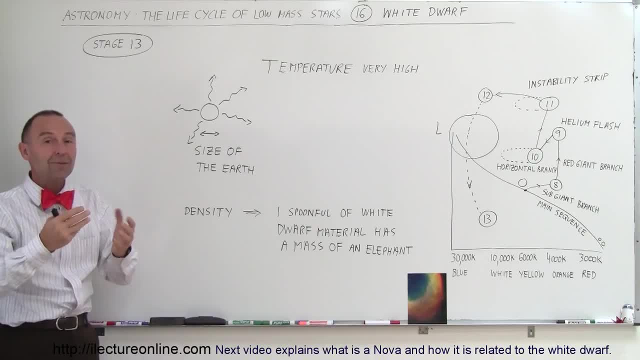 is over 100 million degrees Kelvin. But over time, slowly, the core will cool down and the temperatures will slowly decrease. Nevertheless, the surface temperature of these white dwarf stars are still in the hundreds of thousands or millions of degrees, putting out enormous quantities of UV radiation. How big are these? Now? what's left of the core of the star? it has not collapsed to the size of a regular planet. For example, the diameter of a typical white dwarf is no bigger than the size of the Earth. Yet it contains the mass of hundreds of thousands- well, not necessarily hundreds of thousands, but tens of thousands- two hundreds of thousands times the mass of the Earth, Typically speaking. 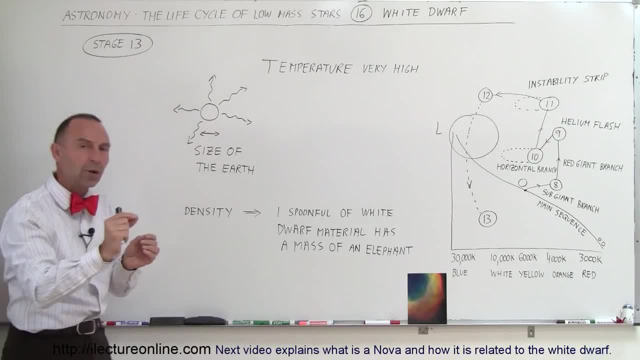 the density of white dwarf material is so dense that if you take one spoonful of material off the surface, it would have the mass of an elephant on the Earth. Typically speaking, the density of a white dwarf is roughly 75,000 times the mass of a white dwarf. 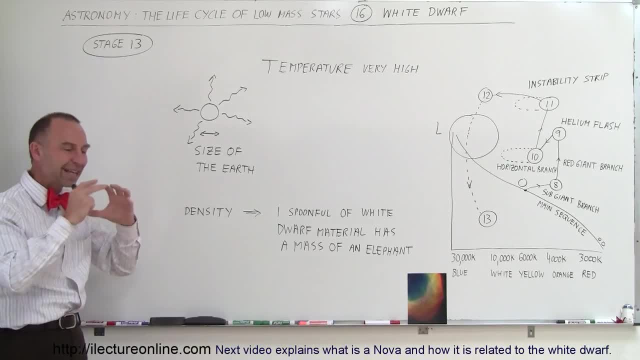 Enormously dense material packed together, almost pure carbon. Carbon is a very plentiful material in the universe because it's being generated by all the stars that reach their red giant stage. Their whole core will fill with carbon and when the rest of the star 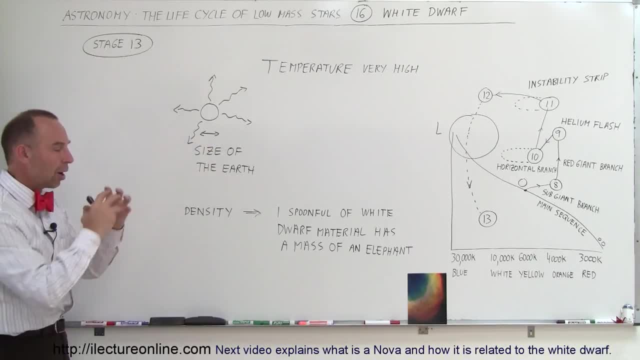 blows away with the planetary nebulas disappearing. all that's left of the star is the center of the star, the core of the star, which is just a ball of very hot carbon. Now, how big can that white dwarf be? Well, a very smart astronomer named Chandrasekhar has actually 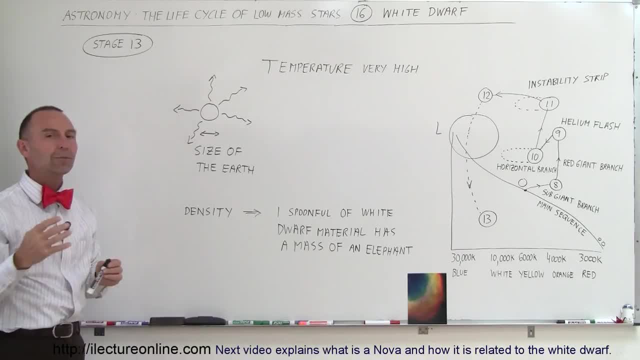 calculated that the maximum mass of the star is 1.4 times the mass of the sun. So the maximum mass that a white dwarf can have is equal to 1.4 times the mass of the sun. What happens when it's bigger than 1.4 times the mass of the sun? And that's what happens to these. 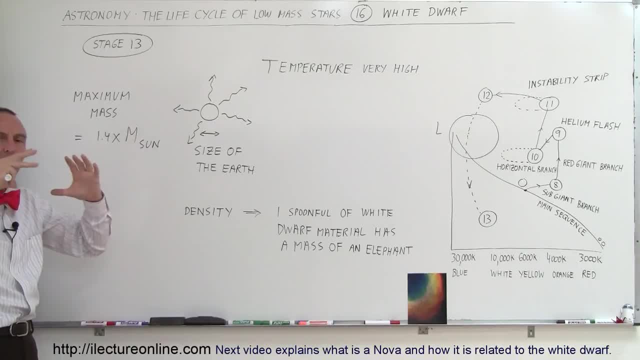 very large stars. A very large star ends up in a white dwarf stage, But somehow the mass of the white dwarf stage that rests the core of the star that's remaining if that exceeds 1.4 times the mass of our current sun. well, the balance between the 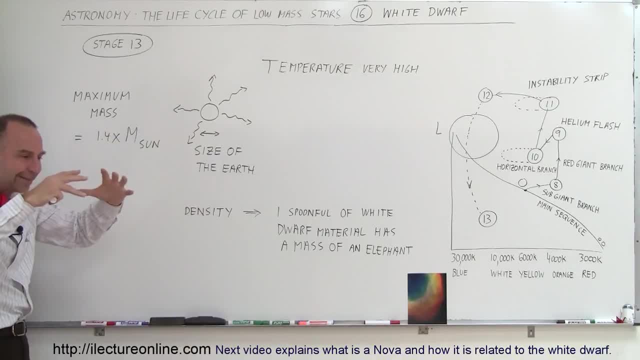 gravitational forces pushing the core ever so tight and the repulsive forces of the electrons pushing back that balance will be overcome by the gravitational forces. It will overcome the repulsive forces of the electrons. It will squeeze the white dwarf even tighter. So as long as the mass does not exceed 1.4 times the mass of the sun, that will not. 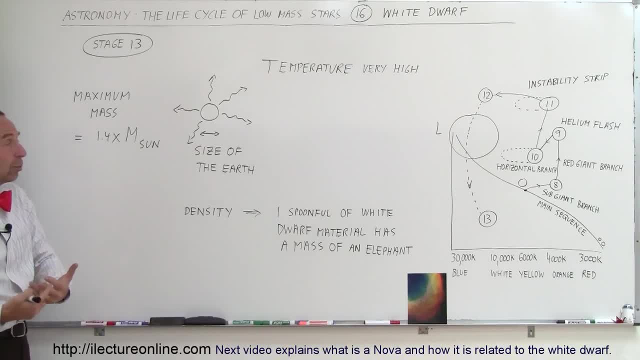 happen, And so the white dwarf typically, for most stars, especially like our sun, which only starts with one times the mass of the sun, it could never have a white dwarf remnant that is bigger than that. So therefore, most white dwarfs will always remain as white dwarfs in the universe, and slowly over the billions. 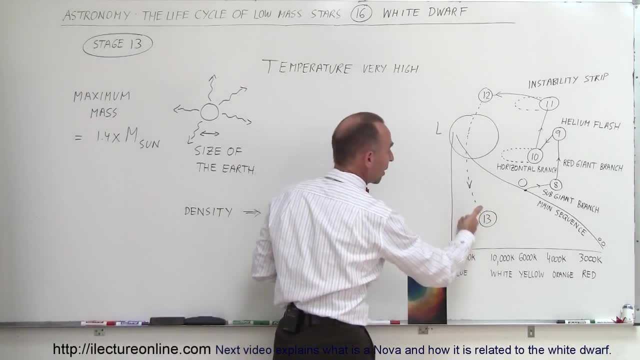 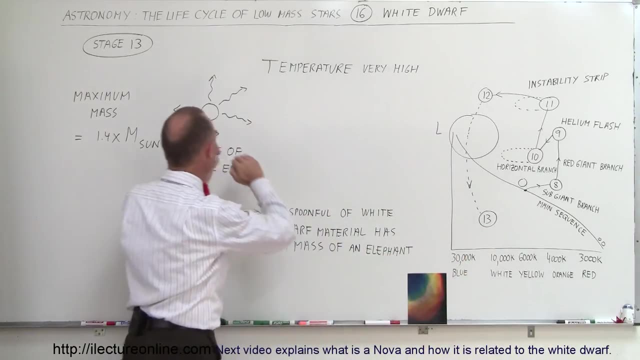 of years cool down. Where do white dwarfs appear on the H-R diagram? Well, down here, because they're not very luminous. They're very hot, but they're not very luminous because they're so small. the surface area of these white dwarfs are so tiny. here you can take a look at it. 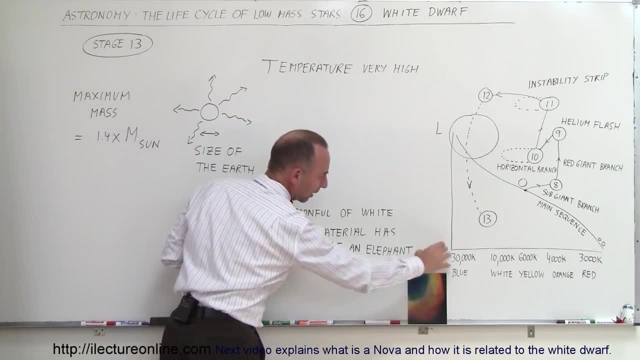 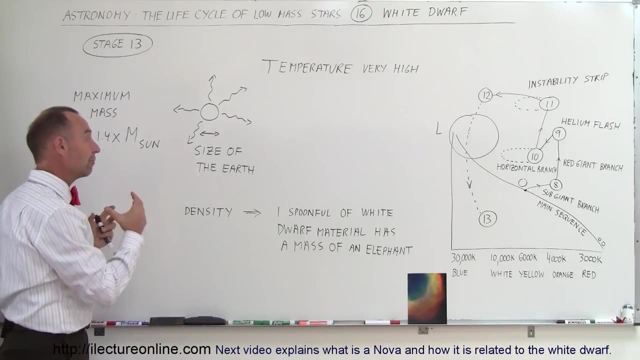 that is, a white dwarf remnant with the outer layers, the planetary nebula, slowly fading away in the ring nebula. so you can see, these are very, very small objects, very hot on the surface but very small, and they're not very luminous. that's why they appear so low on the hr diagram and of 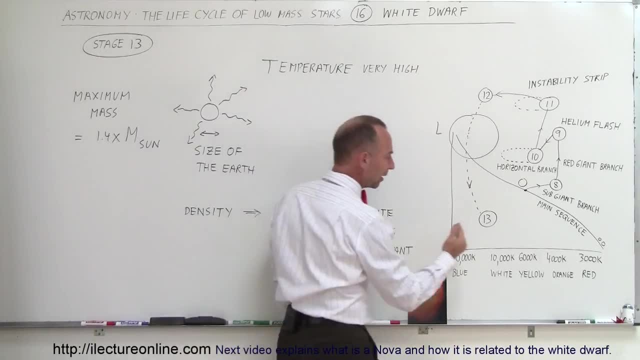 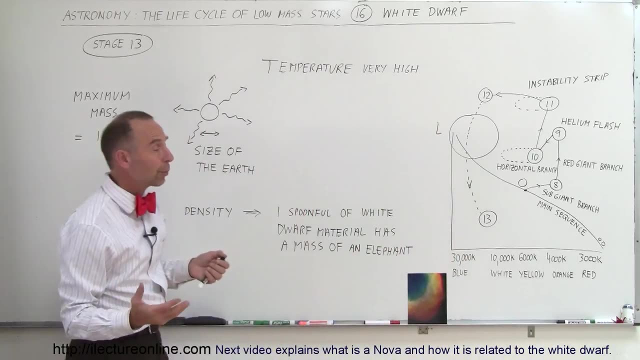 course, over time, as they cool down and they give off less and less energy, they will slowly move to the right on the hr diagram. of course, in the entire history of the universe- the 13.78 billion years of universe is old and that stars have been in existence that have slowly turned into. 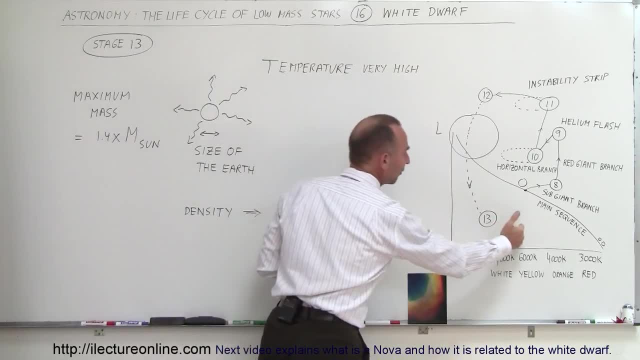 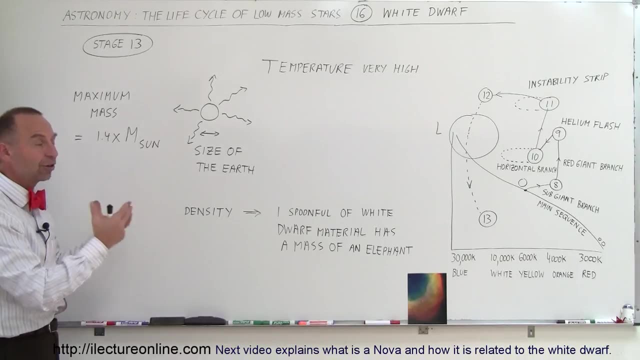 white dwarfs. none of them have gotten to the point where they're no longer visible because it takes so many billions of years for them to cool down. so all the white dwarfs that have ever been formed in the universe are still there, visible to us, just hard to find, because they're 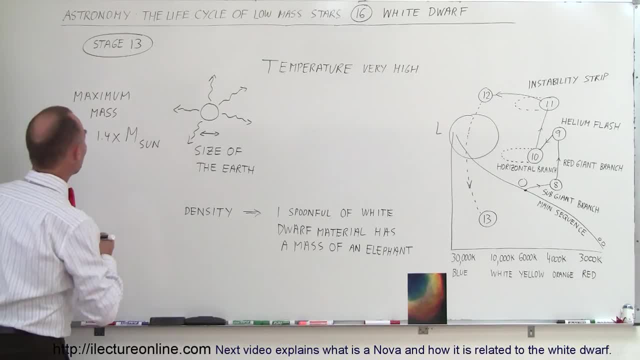 so tiny and so small. now, let's see here, since this is a very special limit, let's write down the name of the white dwarf, which is the white dwarf, which is the white dwarf, which is the, and dthe last one was part of theaturic universe, which is part of theatory, which is part of theatory. 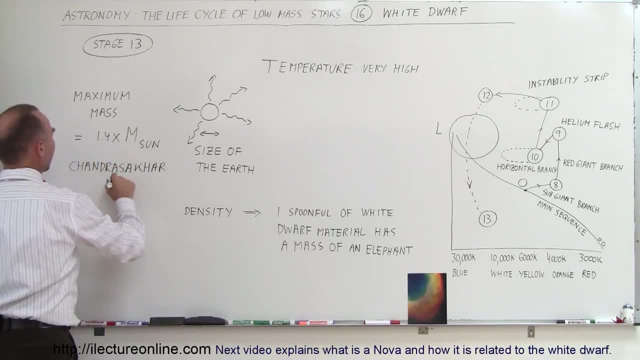 limit. this is known as the Chandrasekhar limit, and that is the ultimate size limit for any white dwarf, which is 1.4 times the mass of the sun. and that's where all the stars that we know of, about 99.9 of all the stars, with a very small percentage of stars that do not go to this final end stage.